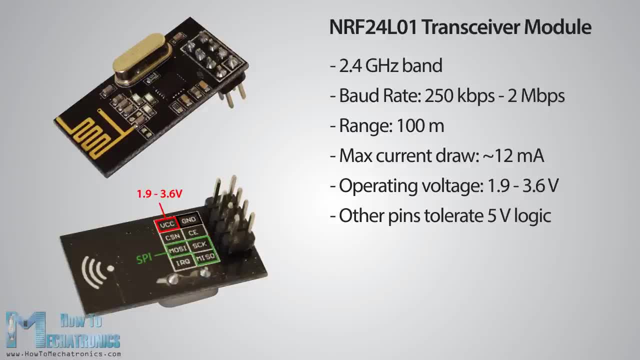 using any logic level converters. Three of these pins are for the SPI communication. The other two pins are for the power consumption. They need to be connected to the SPI pins of the Arduino, but note that each Arduino have different SPI pins. The pins CSN and CE can be connected to any digital pin of the Arduino board and they 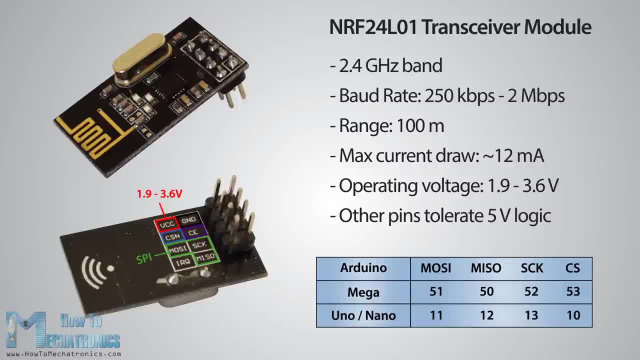 are used for setting the module in standby or active mode, as well as for switching between transmit or command mode. The last pin is an interrupt pin which doesn't have to be used. So once we connect the NRF24L01 transceiver module to the Arduino board, we will have a 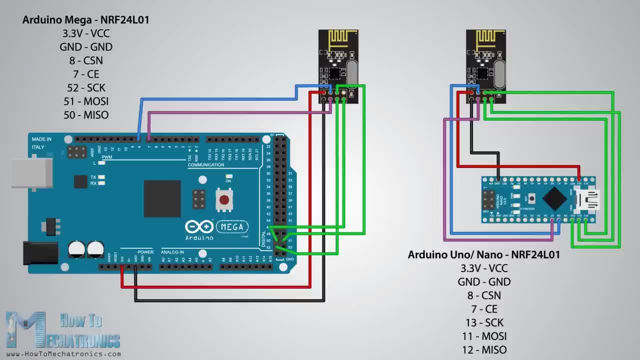 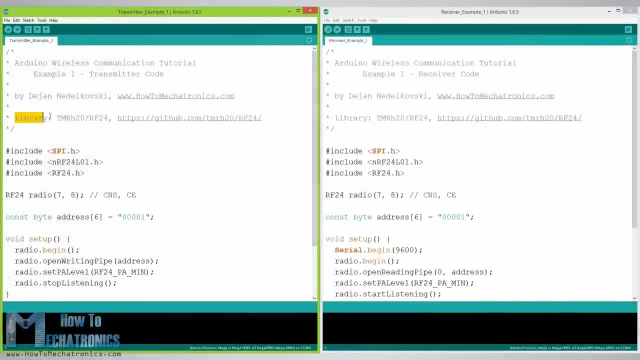 very simple and easy way to connect the module to the Arduino board. We are ready to make the codes for both the transmitter and the receiver. First we need to download and install the RF24 library and make sure you have the correct one. You can find the download link on the website, article. 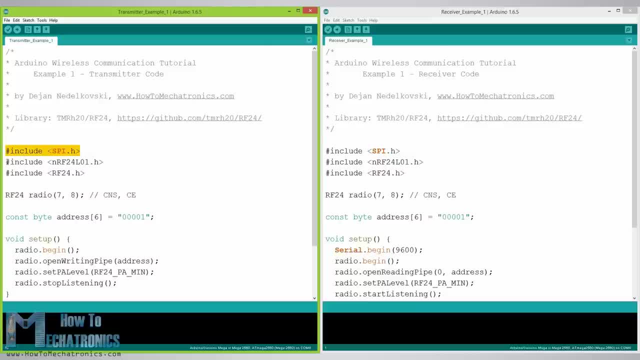 So we need to include the basic SPI and the newly installed RF24 libraries and create an RF24 object. The two arguments here are the following: The first argument is that we need to install the RF24 library. We have the CSN pins and the CE pins. 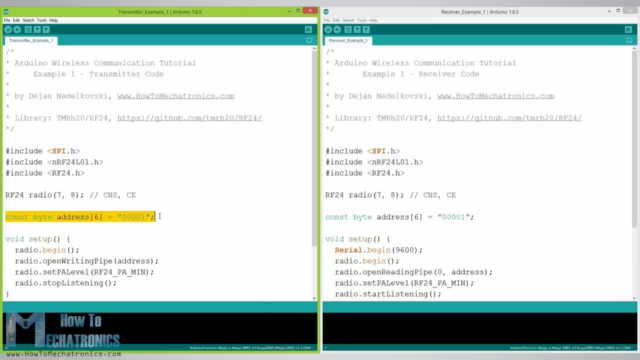 Next, we need to create an array which will represent the address or the so-called pipe through which the two modules will communicate. We can change the value of this address to any 5 letter string, and this enables to choose to which receiver we will talk. 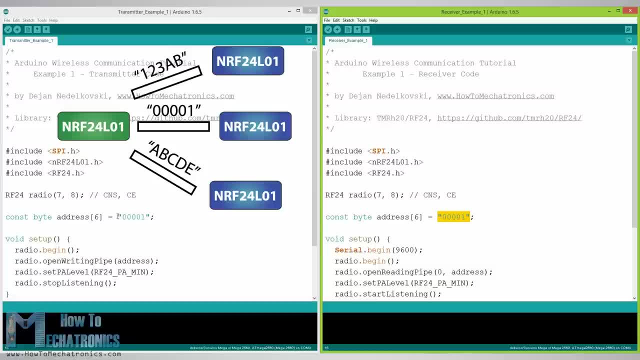 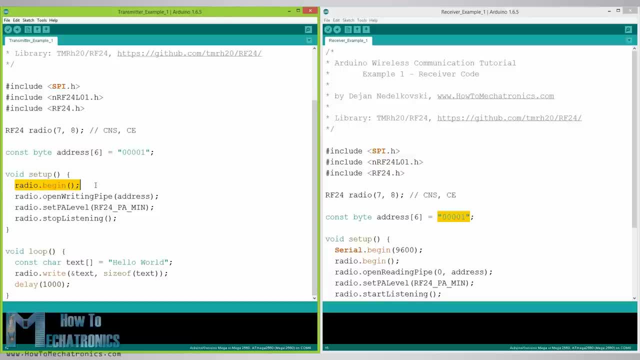 So in our case we will have the same address at both the receiver and the transmitter. In the setup section we need to initialize the radio object: the radio object and using the radioopenWritingPipe function we set the address of the receiver to which we will send data, the 5 letter string we previously set. 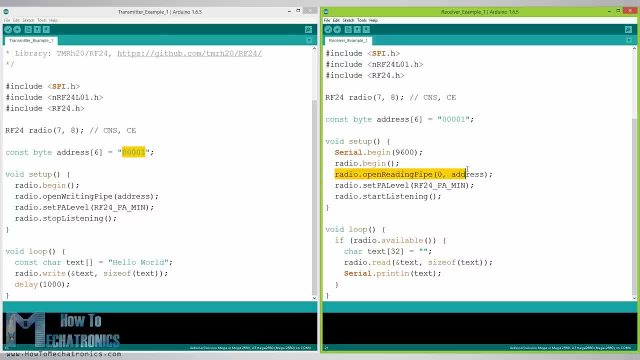 On the other side, at the receiver, using the radiosetReadingPipe function, we set the same address and in that way we enable the communication between the two modules. Then, using the radiosetPaLevel function, we set the power amplifier level. in our case I will set it to minimum value, as my modules are very close to each other. 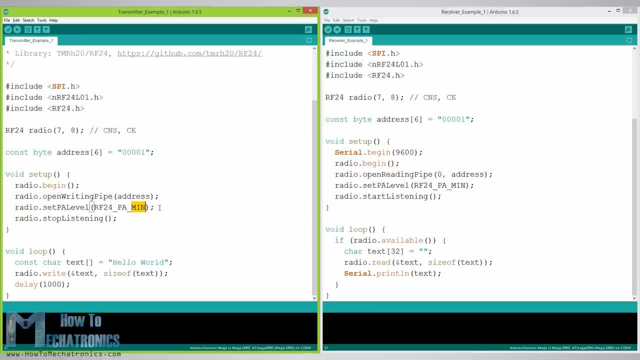 Note that if you are using a higher level, it is recommended to use a bypass capacitors across the ground and the 3.3V of the modules so that they have more stable voltage while operating. Next we have the radiostopListening function, which sets the 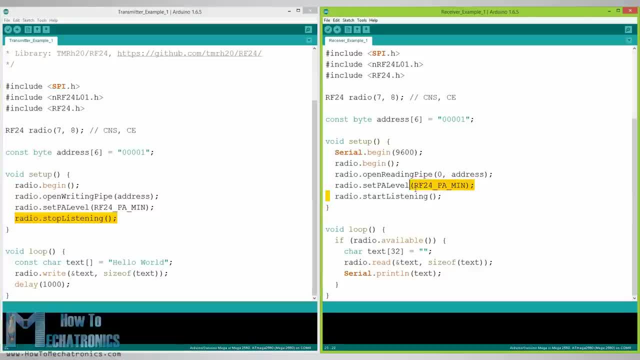 module as transmitter and, on the other hand, we have the radiostartListening function, which sets the module as receiver. In the loop section at the receiver, we create an array of characters to which we assign the message: hello world. Now, using the radiowrite function, we will send the message to the receiver. 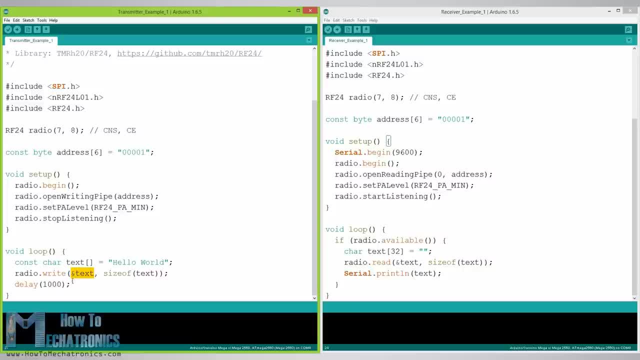 The first argument here is the variable that we want to be sent. by using the & before the variable name, we actually set an indication of the variable that stores the data that we want to be sent. and using the second argument, we set the number of bytes that we want to. 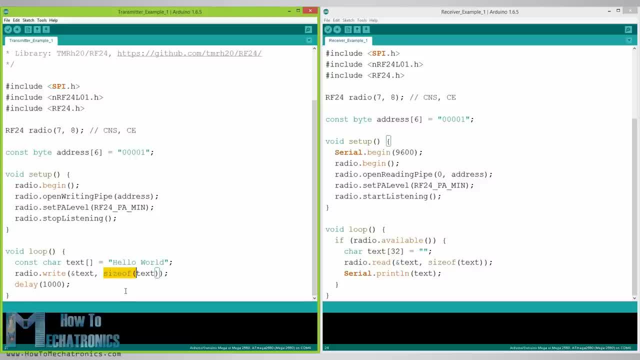 take from that variable. In this case the function sizeOf gets all bytes of the string text. At the end of the program we just add one second delay. On the other side, at the receiver, in the loop section, using the radioavailable function, we check whether there is a message. 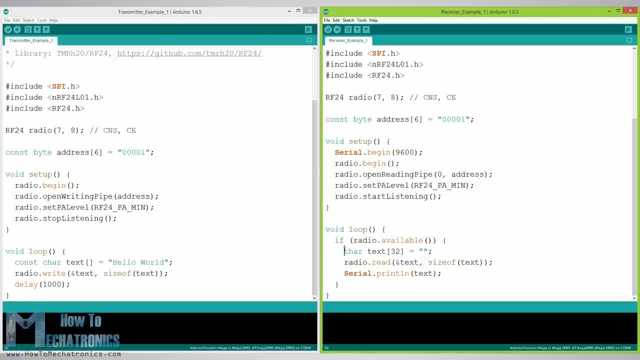 If that's true, first we create an array of 32 elements called text, in which we will save the incoming data. Using the radioread function, we read and store the data into the text variable. At the end, we just print the text on the serial monitor. 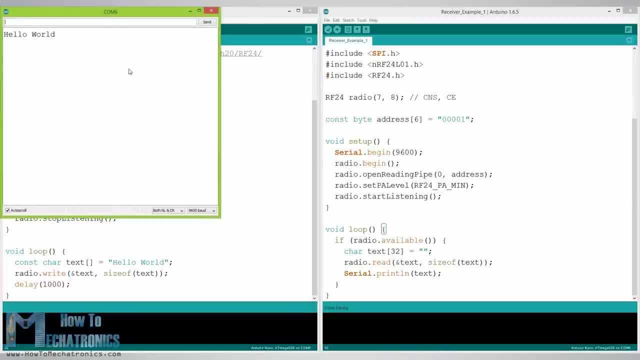 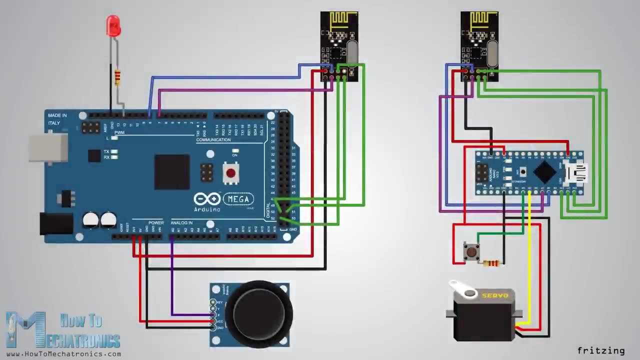 So once we upload both programs, we can run the serial monitor at the receiver and we will notice the message hello world gets printed each second. Next we have the serial monitor, 그렇죠. Next, let's see the second example. 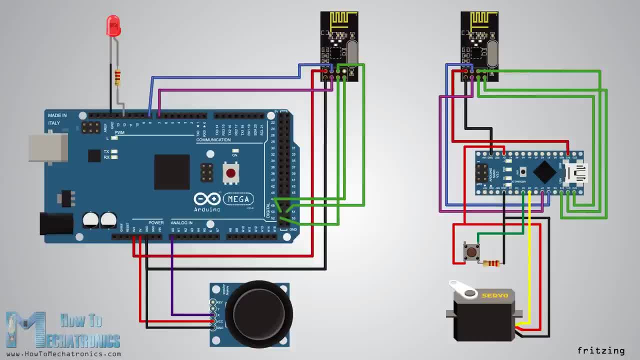 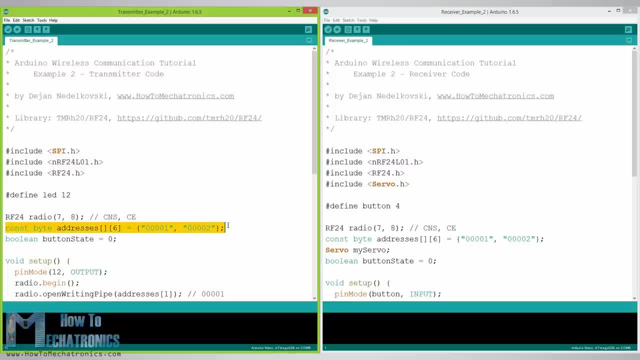 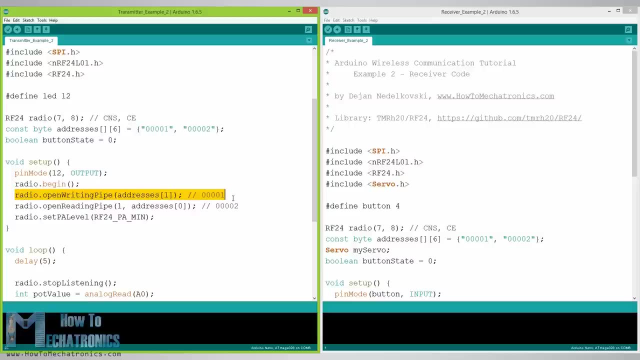 Here is the circuit schematic, and now we will take a look at the Arduino codes. What's different here from the previous example is that we need to create two pipes or addresses for the bidirectional communication bar In the setup section. we need to define both pipes and note that the writing address at 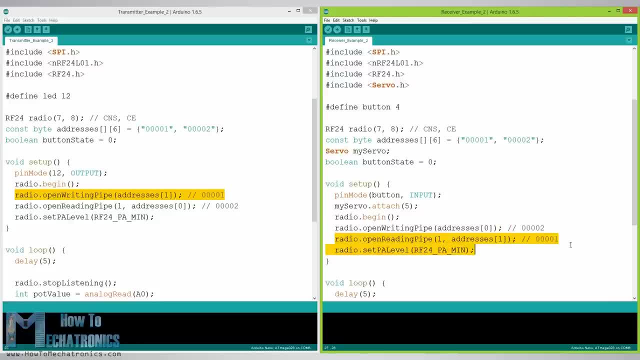 the first Arduino needs to be the reading address at the second Arduino, and vice verse: the reading address at the first Arduino needs to be the writing address. Then inner optimization will take complete control over both pipes. Let's check this out. Both pipes are working. 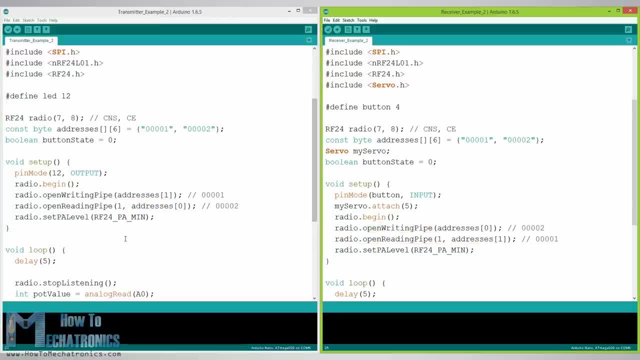 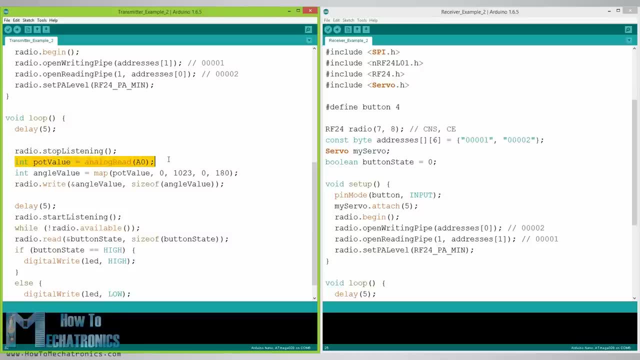 All right, Now I'm going to seven, the weirdest act of doing this right now我在. here. I have another, an argument set and we'll take it as expected. address at the second Arduino In the loop section. using the radio dot stop listening function, we set the first Arduino as transmitter, read and map the. 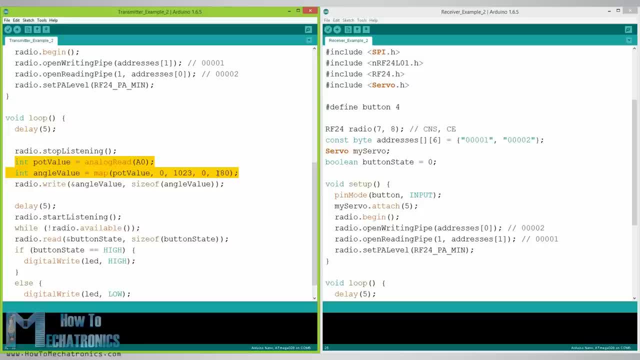 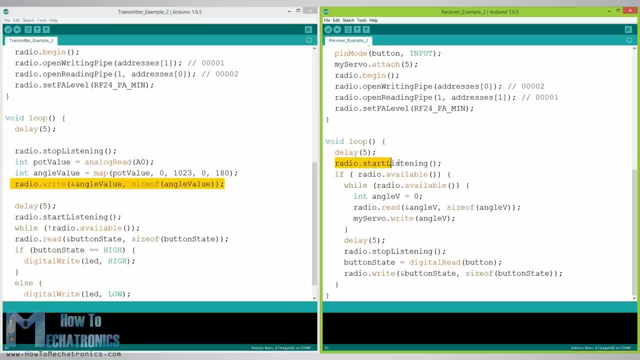 value of the joystick from 0 to 180 and, using the radio dot write function, send the data to the receiver. On the other hand, using the radio dot start listening function, we set the second Arduino as receiver and we check whether there is available data. While there is available data, we will read it, save it to the 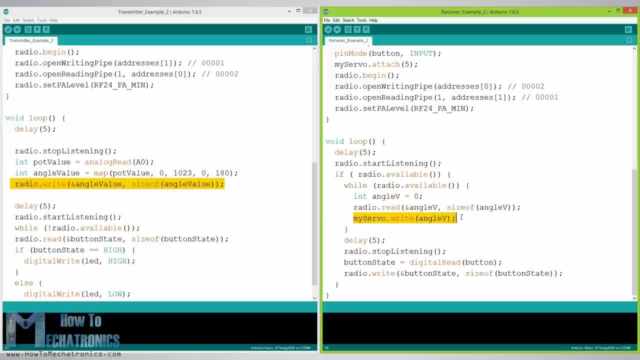 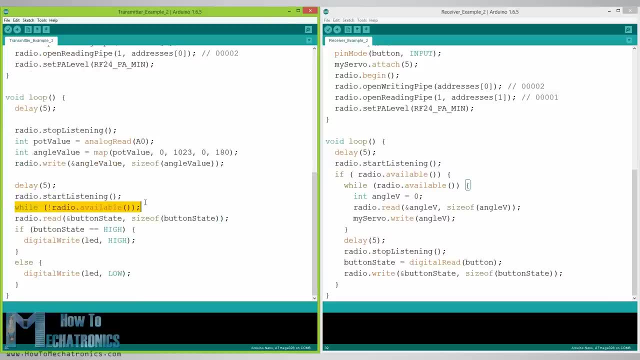 angle V variable and then use that value to rotate the servo motor. Next, we set the first Arduino as receiver and with an empty while loop we wait for the second Arduino to send data, and that's the data for the state of the push button, whether it is pressed or not. If the button is pressed, the LED will light. 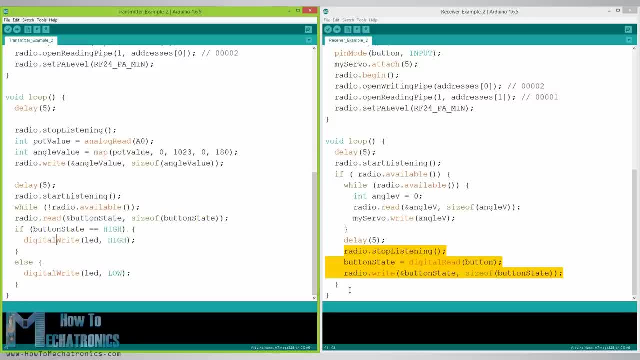 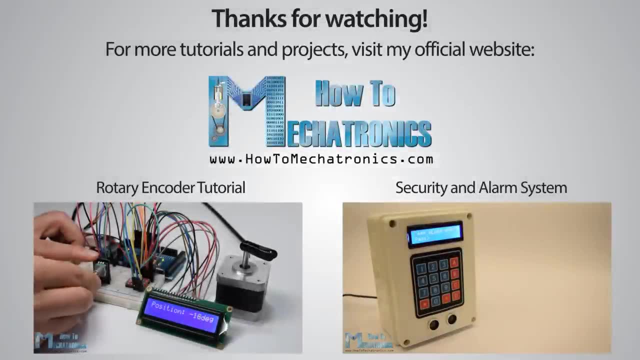 up, So this process constantly repeats and both Arduino are constantly sending and receiving data. That's all. thanks for watching, and for more tutorials and projects, visit my official website, howtomechatronicscom. 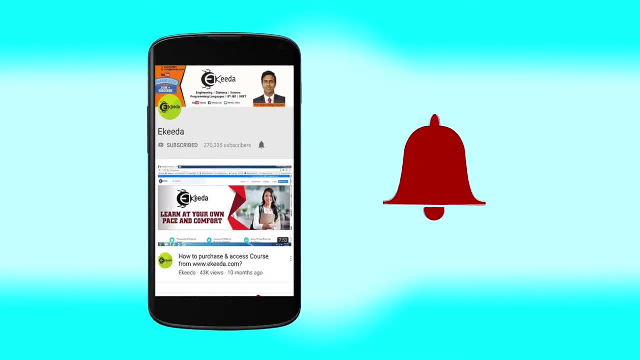 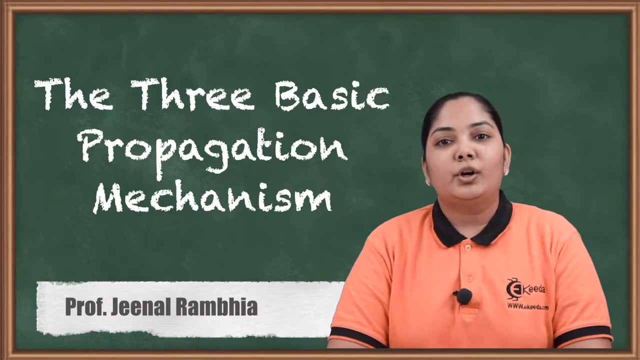 Click the bell icon to get latest videos from eKIDA. Hello friends, in this lecture we will be studying the three basic propagation mechanisms. We all know in mobile radio communication there is a line of sight of path through which the communication takes place. But when there is no line of sight of path, there is still. 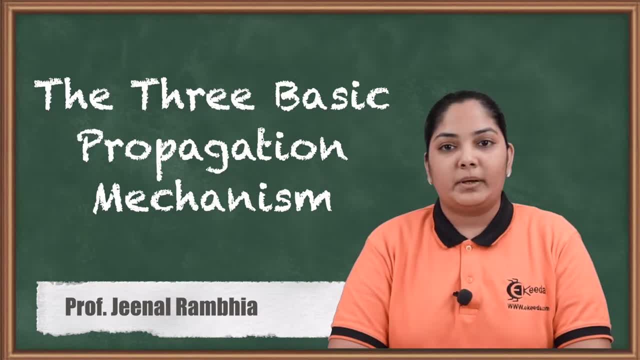 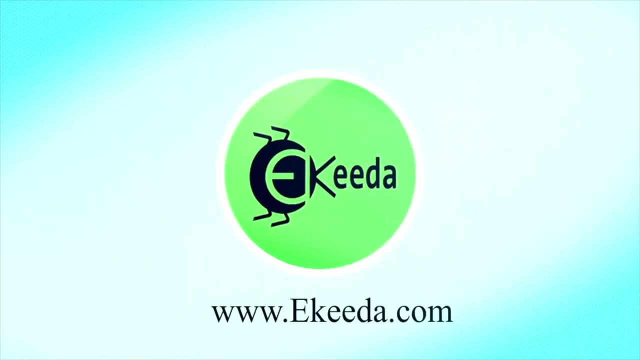 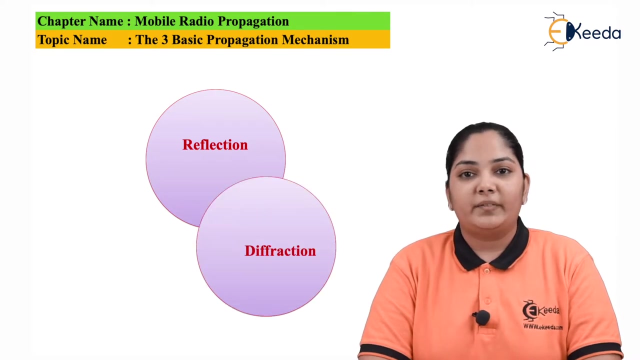 communication possible. And it is possible because of these three methods that are called as reflection, diffraction and scattering. Let us study in this lecture the meaning of all of these three. The first one is called as a reflection. Reflection means that the electromagnetic wave in the mobile communication is impinging on an object And the dimension.